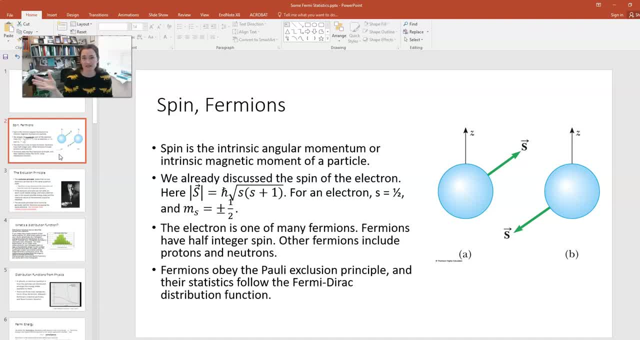 I would think of the charge of a particle or the mass of a particle, just like that. It also has this other property called spin. all right, So this is the angular momentum. Now the spin is quantized for quantum particles. okay. 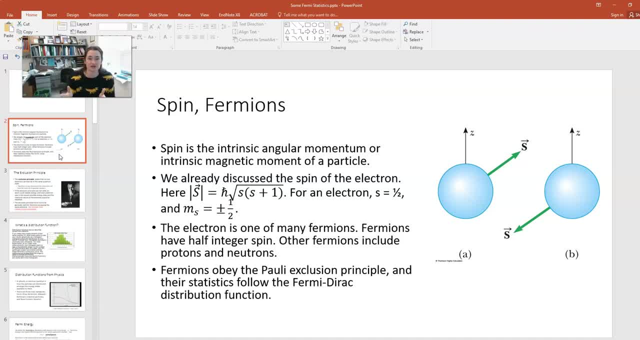 It can't just have any old value, In other words, it's going to have certain discrete values. So that's dictated by the spin quantum number. Now for fermions, and in that class of particles an electron is a fermion. 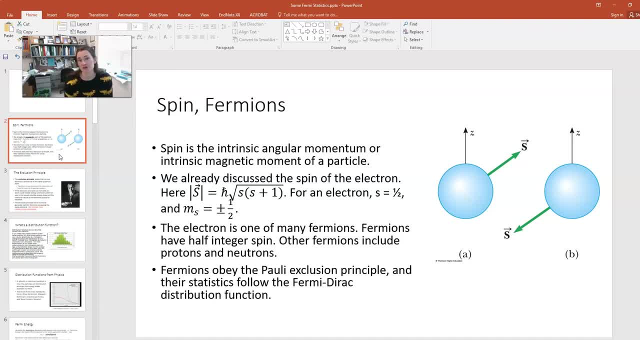 the spin is a half integer. So for an electron, for example, the spin quantum number S is one half. Now we often talk about spin up and down right, And that has to do with how these particles behave in a magnetic field. okay, 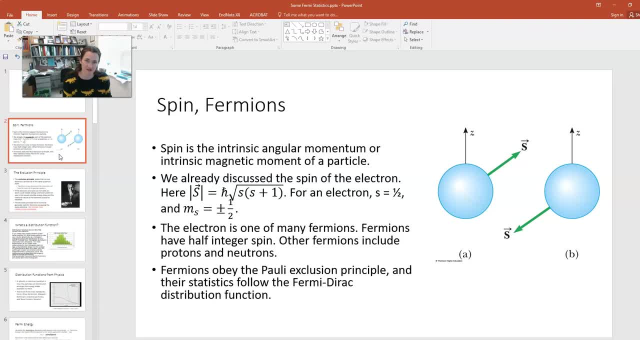 So if you have an intrinsic magnetic moment, dictated of course by the fact that you have an intrinsic angular momentum, then the particle could either align with that magnetic field or be anti-parallel to the field. okay, And this corresponds to spin up and spin down particles. 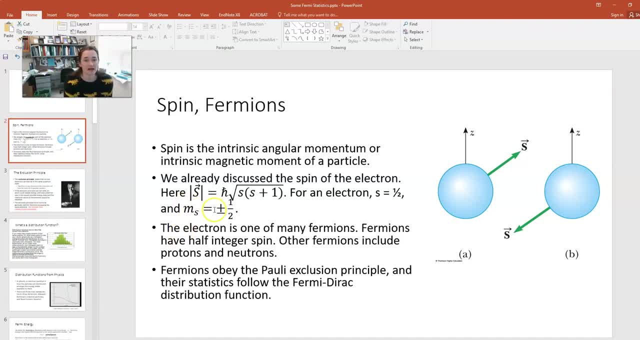 And the way that we quantify, that is, with the magnetic spin quantum number M sub S, whose value for an electron is either plus or minus one half. So plus one half corresponds to spin up, minus one half is spin down. So the electron, as I said, is one of many fermions. 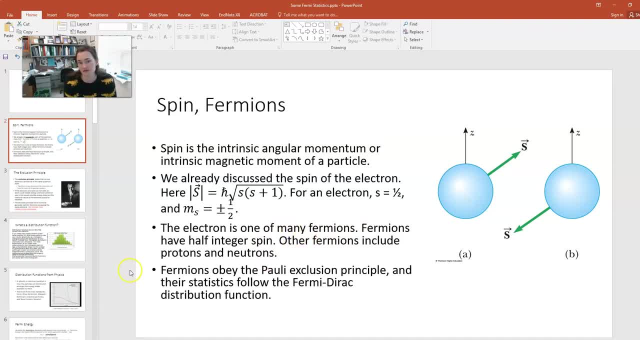 Fermions have half integer spin. Other fermions that you may have heard of include protons and neutrons, which are also present in atoms. Now, what's special about fermions is that they obey the Pauli exclusion, and that means that they are dictated by a set of statistics. 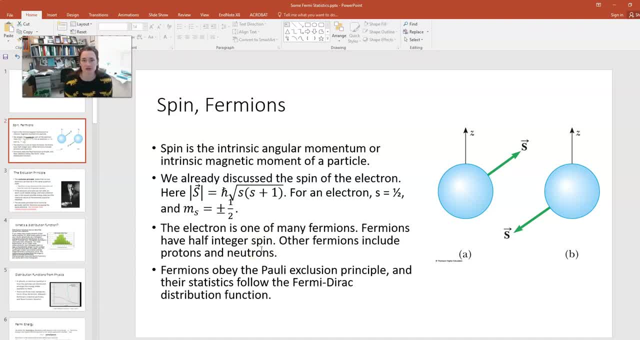 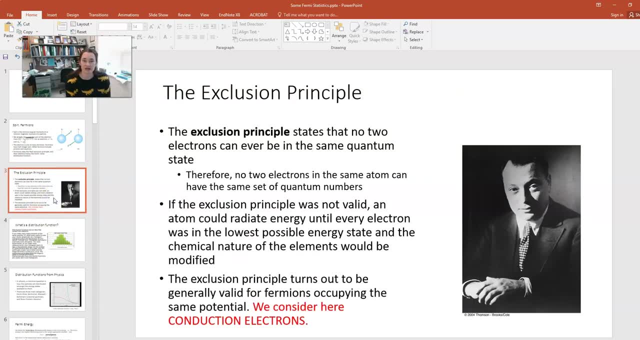 that are distinct from other types of particles like bosons or classical particles. So let's remind ourselves what the exclusion principle is. The exclusion principle states that no two fermions that are in the same potential can have the same set of quantum numbers. So what this means for, for example, electrons in an atom. 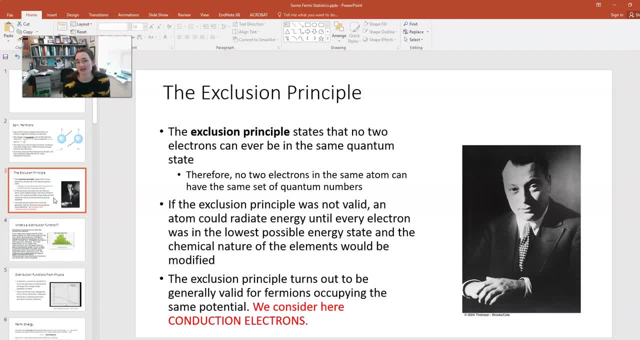 is that no two electrons in the same atom can have the exact same set of quantum numbers, And if that's the case, then the exclusion principle states that no two electrons in an atom can have the exact same set of quantum numbers. this weren't valid. what would happen is that all the electrons to be in their 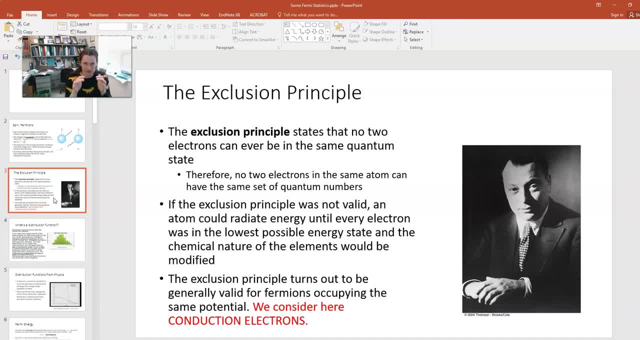 lowest energy state would radiate away until they were in the lowest ground state, but that's not what happens, and so that dictates the structure of our periodic table, for example, amongst other things. now, in this case, I'm not focusing in on what going on with electrons within an atom. I'm going to talk today. 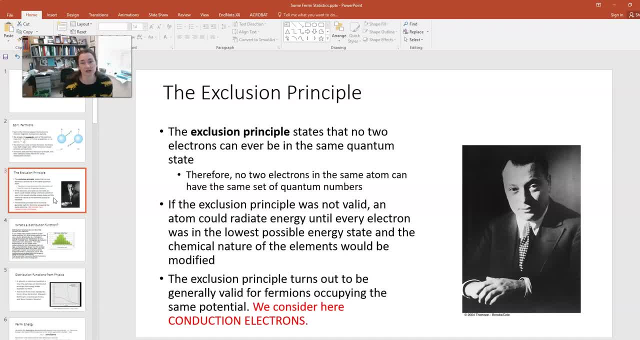 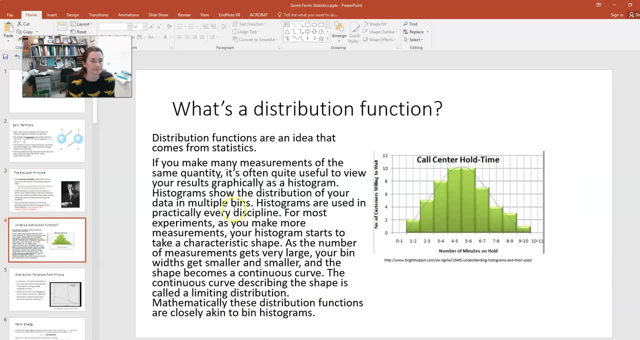 about the free electron C or the free electron gas that's present for conduction electrons in a metal lattice. okay, so to talk about this, I'm gonna have to talk about the fermi Dirac distribution function, so I thought it might be worthwhile to remind you of what a distribution function is before I 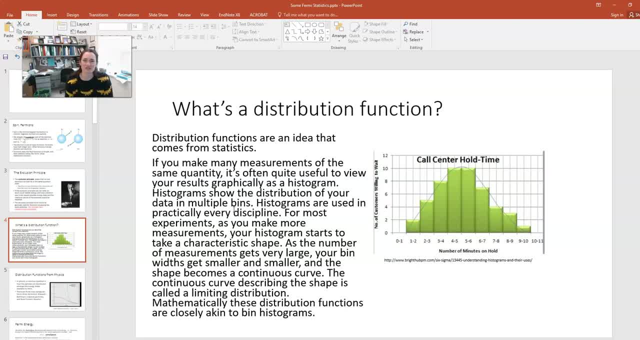 do anything else. okay, so distribution functions are is an idea that comes from statistics. so basically we do a lot of histograms and distribution functions in a lot of different fields. they start off say: maybe as a histogram here this is, for example, call center whole time versus number of minutes. 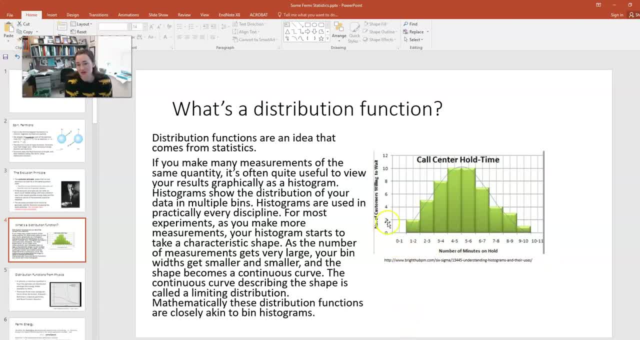 for a business. okay, so you can see here lots of different folks like to use histograms and distribution functions. basically, the idea is that you have so, for example, here for call center, whole time it's the number of customers willing to wait versus the number of minutes they're put on hold. 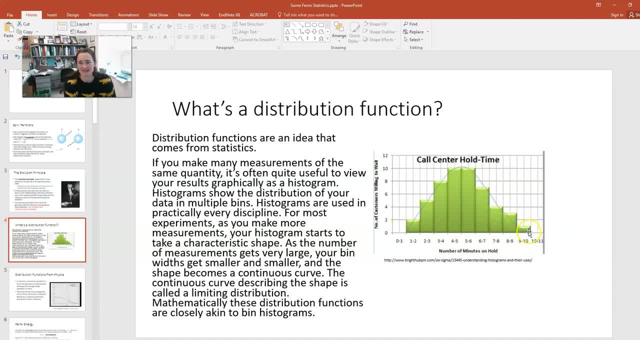 right. so how many customers are actually willing to wait nine to ten minutes? it's not very much right, all right. so, um, what's going on with the statistics that we're talking about today is in physics. we're really interested in how particles distribute their energies within a 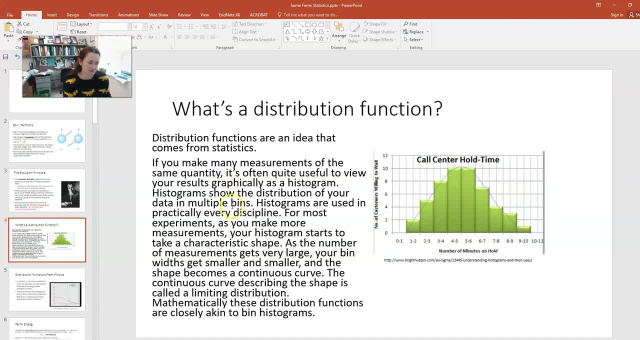 system. so how many particles might have x amount of energy, how many particles might have y amount of energy? and if you have a big collection of particles and you plot their energies right, how many particles will you find in a given energy range? and so that's the kind of 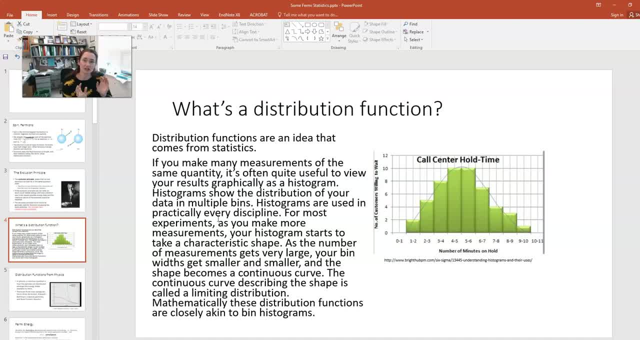 histogram that we're plotting. now, when you're looking at large collections of data, what happens is your bins, how wide your bin is there, and that then histogram gets narrower and narrower and it starts to look- your function starts to look more and more continuous. so you can see here it's done a little bit in. 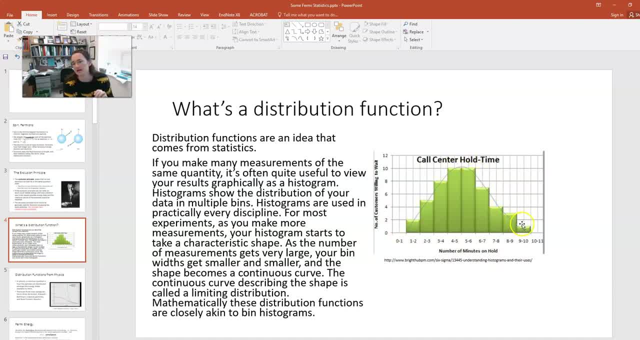 this image. they're plotting out where the top of that bin is for each one, and you can see that it starts to look like a continuous function, and the more data you got right, the more continuous it would look. so this is the distribution function. so you can think in your head: okay, I've got histograms and then as it, 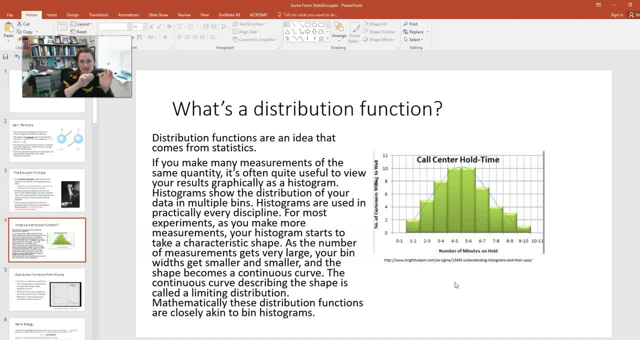 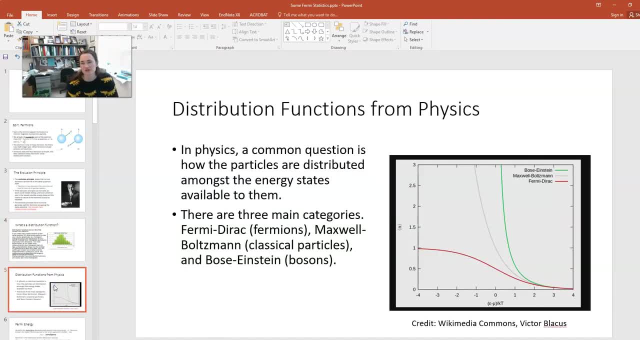 gets more and more data and my bins get. my bins get smaller and smaller. I've got distribution functions, but they do kind of the same thing. now, what distribution functions do we have in physics that do these sorts of things? well, there's three common classes of particles that you learn about in statistical mechanics. 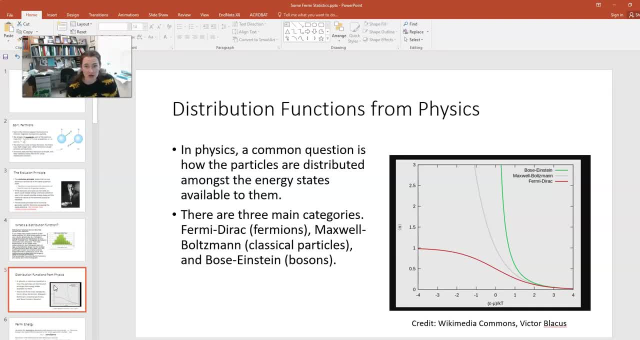 those are your bosons, your uh, fermions, and then your classical particles, and to describe classical particles, you usually think of ideal gases, right? so those are the three classes of particles. and so how are the energy states for a bunch of these types of particles? how are they distributed, right? how is it? how does it go for? 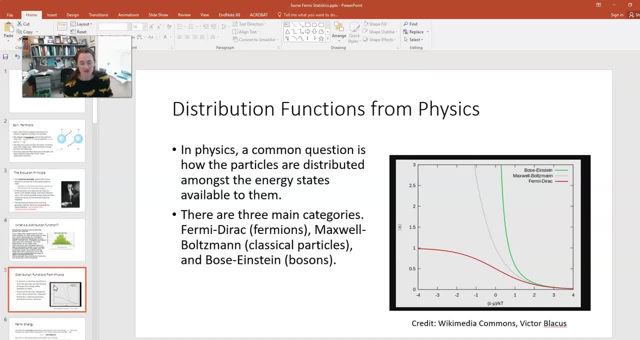 classes of particles with different temperature ranges. all right, so to do that, we have three classes of statistics: Fermi Dirac statistics, Maxwell Boltzmann statistics, those describe classical particles and Bose-Einstein statistics and those describe bosons. and we're not going to talk about Maxwell-Boltzmann or Bose-Einstein today. I'm going to focus in 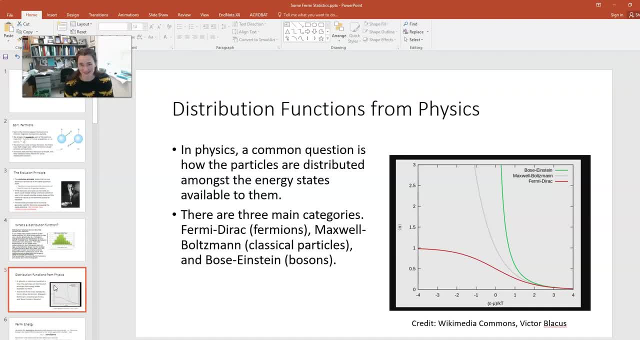 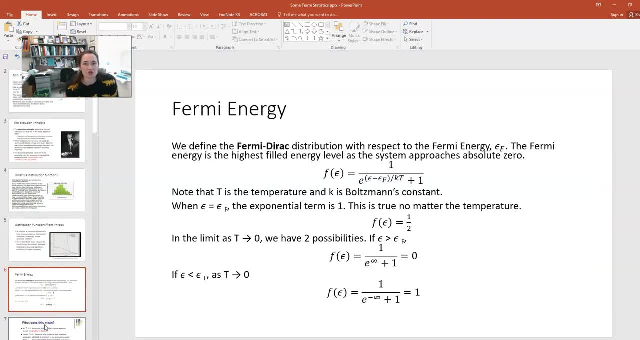 on Fermi Dirac, because those describe fermions right and that's what we're interested in for the conduction electrons. so what is the distribution function for fermions? what is the Fermi Dirac distribution function? here it is shown. the function that I'm showing here is f of epsilon. here epsilon represents the energy that a particle might get. is actually the energy which the particle might? eGif estar. 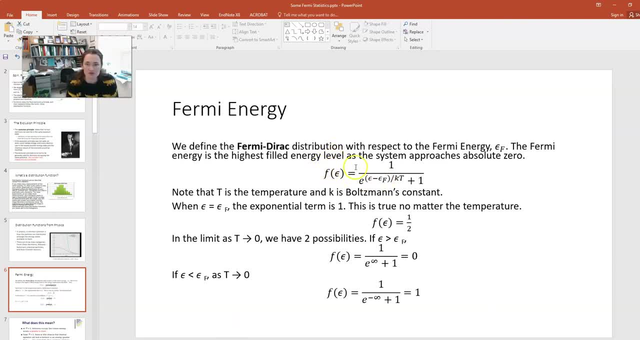 EF checked, which is the universe. So if EF is aren't going to, pela Er Klian represents the energy that a particle might have. F of epsilon is equal to 1 over e, to the minus epsilon, minus the Fermi energy divided by K, T plus 1. now, 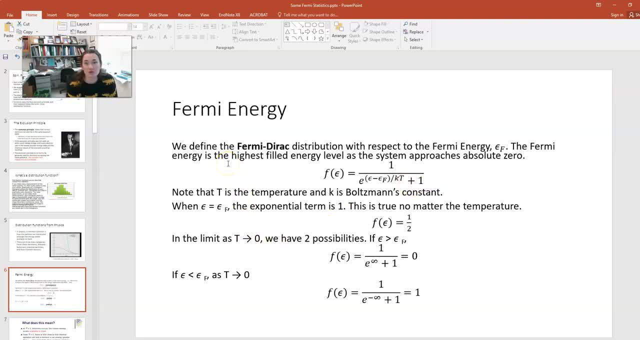 here K is Boltzmann's constant, which in SI units is 1.381 times 10 to the minus 23 joules per Kelvin. right epsilon sub F is the Fermi energy. we're going to be talking about a lot about the Fermi energy here in a second and, of course, T. 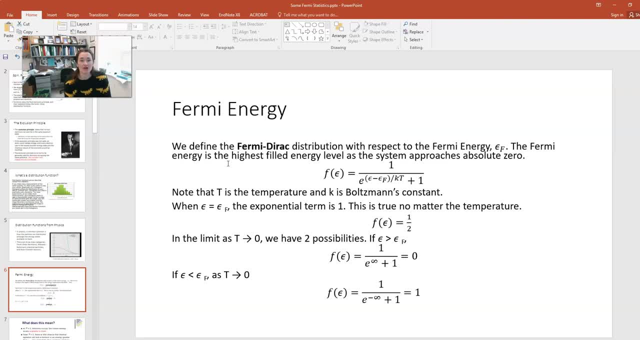 is the temperature. okay now, the Fermi energy is a very important energy when describing fermions. all right, what it is in a nutshell- and we'll talk about this more- is the maximum possible energy that a particle can have when that system of fermions is at absolute zero. okay, so that's the highest occupied energy state. 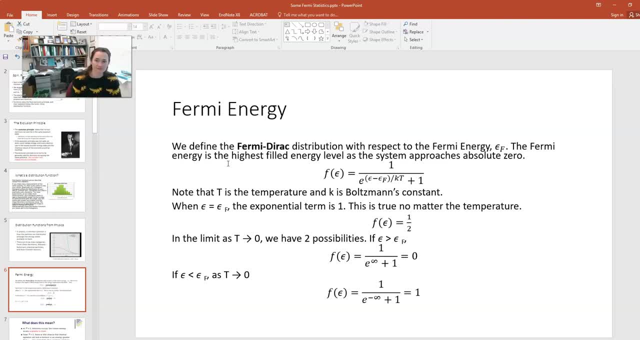 at absolute zero for a system of fermions. okay, now how does this function describe that? let's get into this. okay, so if you have a particle, energy is equal to the Fermi energy and then you solve for what that's like here in this Fermi direct distribution function F of 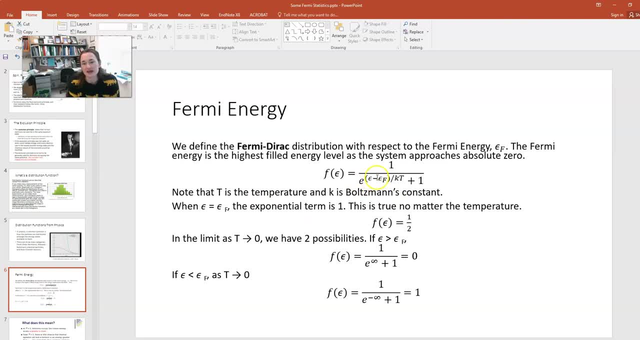 epsilon, then what would happen is: in the e to the epsilon minus Fermi, energy over K T term e would equal e Fermi and then you'd have e to the zero. there in the bottom e to the zero is one, so then you would have one over one plus one which 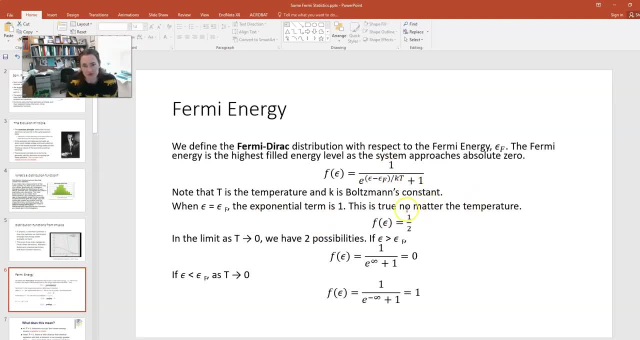 is one half. so if the particles energy equals the energy, then that value of your Fermi direct distribution function is one half, and that's true no matter the temperature. all right, so that's always true. now, what happens as you take T to zero, right? what happens is you shrink. 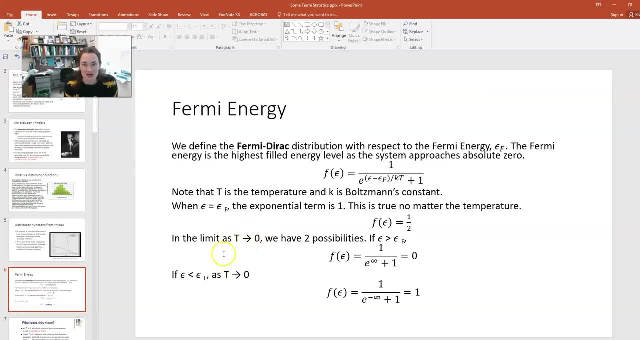 that temperature down towards zero. okay, well, we've got two possibilities. first of all, if you're looking at a particle whose energy is greater than the Fermi energy, then you've got over here, one over something e to the something divided by zero, right? so basically your. 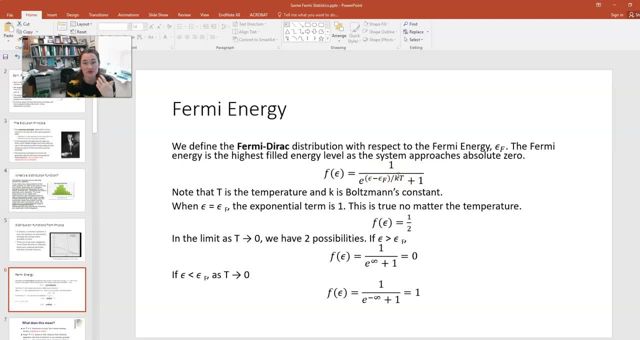 term in your exponential. there it goes to infinity. so you have one over e to the infinity, plus one right that goes to one over infinity which is zero. all right, so if your particles energy is greater than the Fermi energy, as T approaches zero, your Fermi direct distribution function equals zero. and 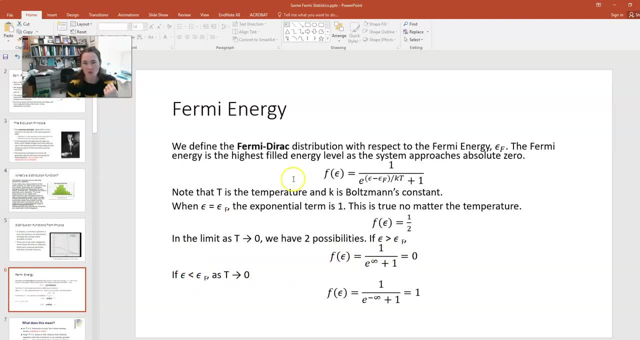 thatijk the function f of theuches, and I'll fill that in here. what do we have? what does that mean? I'll change that number to one. well, if our F goes to zero and T goes to zero, then that means there aren't any particles in that energy state, which means that if the energy is greater than 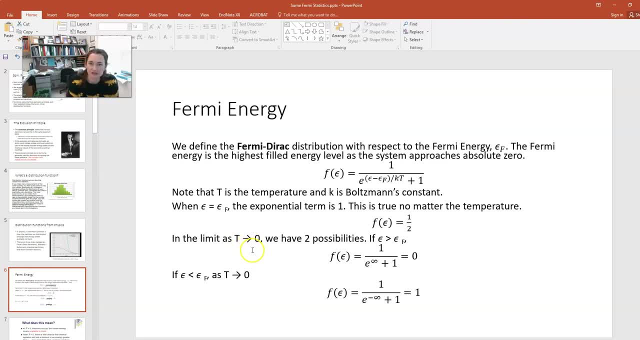 the fermi energy Right Thehydrama have an energy greater than the Fermi energy as t approaches zero. All right, let's look at what happens if the energy epsilon is less than the Fermi energy as t approaches zero. okay, In that. 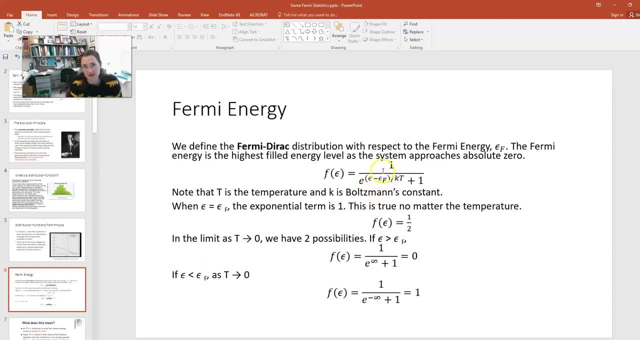 case epsilon minus e Fermi, right, the Fermi energy would be a negative number, right? In that case you have e to the negative number divided by zero. So that means it approaches negative infinity, right? So then you have 1 over e to the minus, infinity plus 1.. Well, e to the minus. 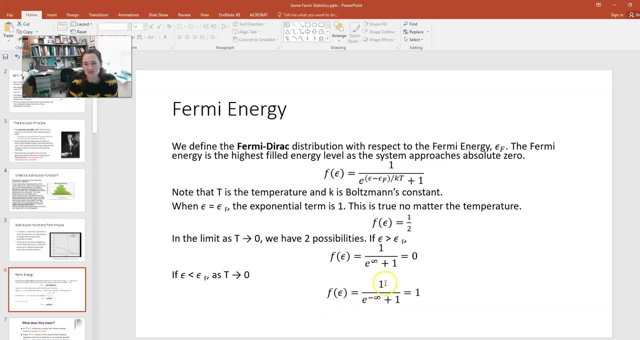 infinity is zero, right? So that means that you have 1 over 1, which is 1.. So basically, if the energy of the particle is less than the Fermi energy as t approaches zero, then you have e to the minus infinity, plus 1.. So that means that you. 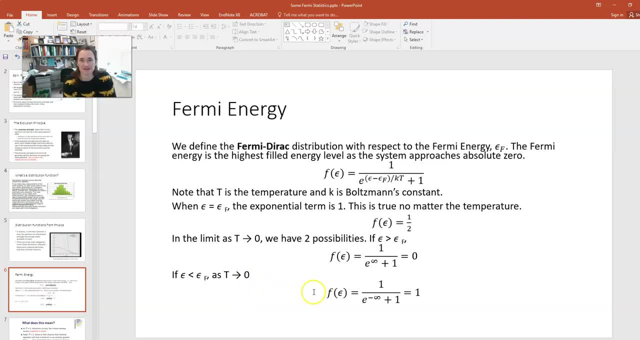 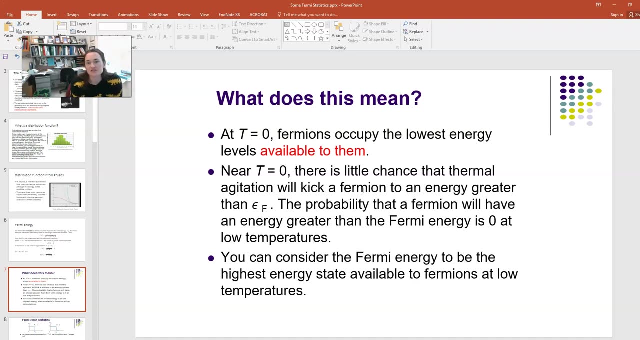 have 1 over 1, which is 0, then that's definitely an occupied state, right? It's occupied with a probability of 100% 1.. So what this means is that if you have zero Kelvin, right, Fermions are. 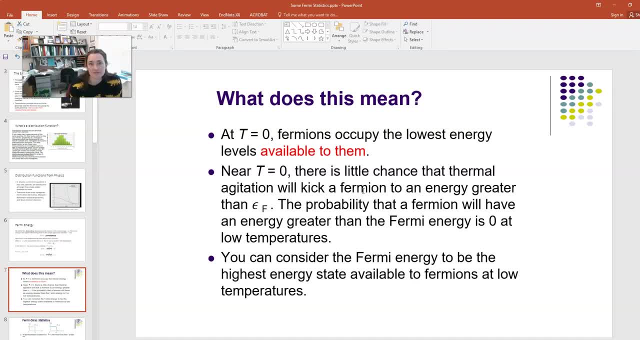 going to occupy the lowest possible energy states available to them. As they chill down, cool off, they're going to be in the lowest possible state that they can get. At near zero Kelvin, there's little chance that they're going to be in the lowest possible state that they can get, So 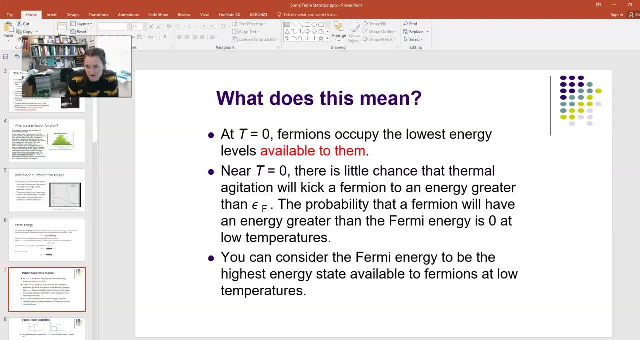 you're going to have thermal agitation taking a Fermion up to an energy greater than the Fermi energy right. So that means that the probability that a Fermion will have an energy greater than the Fermi energy at zero Kelvin is zero right. So you can consider the Fermi energy to be the 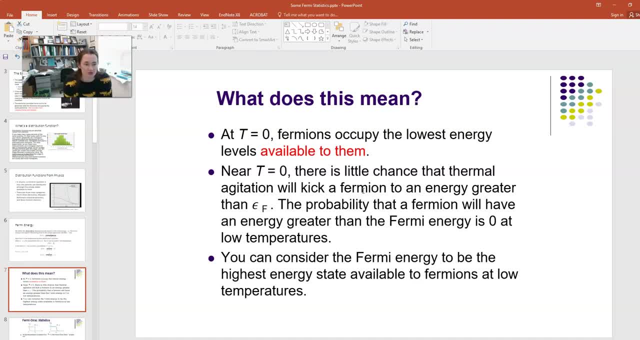 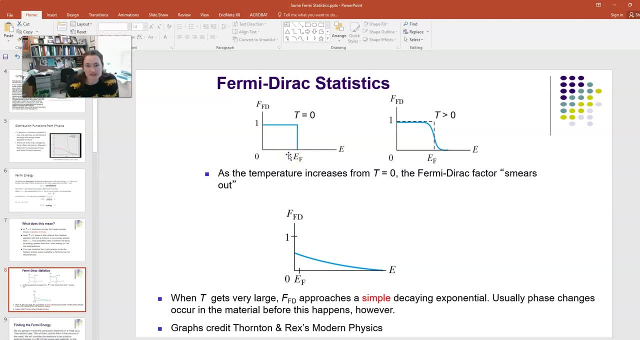 highest energy state available to Fermions at low temperatures. So what does the Fermi-Dirac distribution function look like? Well, if you're at zero Kelvin, it looks like a step function okay. So if you're at zero Kelvin, it looks like a step function okay. So if you're at zero Kelvin. 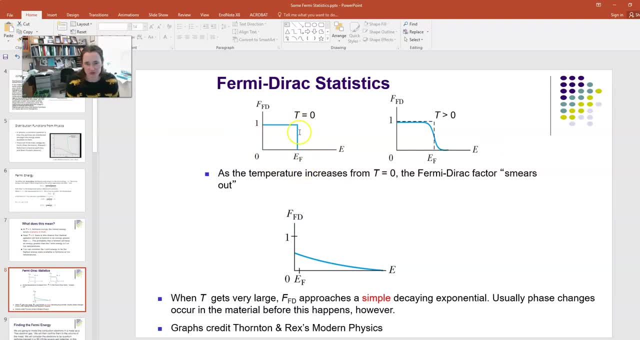 you have this step function in blue and the cutoff is the Fermi energy. here, at T is equal to zero. So basically, the Fermi-Dirac distribution function is one for energies less than the Fermi energy and at zero if it's greater than the Fermi energy. Okay, now what happens if the 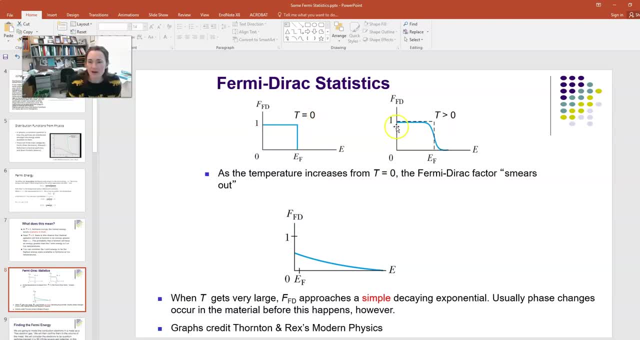 temperature is greater than zero. Well, what happens is it gets rounded off from the step function. So you have sort of a rounded off step for T greater than zero. Now, as we said said, if the energy is equal to the Fermi energy, then the distribution there is one-half, no matter. 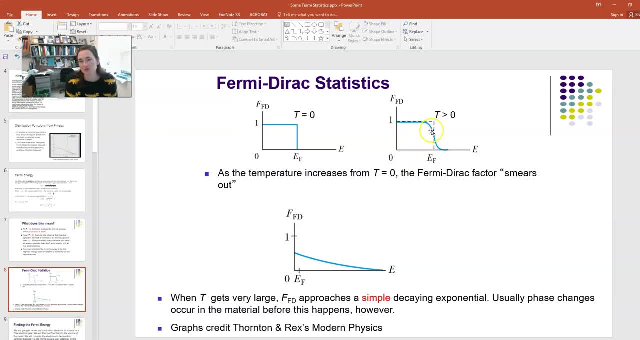 the temperature. So you can see that right here, this blue line right, which represents the distribution function for a greater temperature, intersects the dashed box line right. And where does it intersect it? At one-half okay. So that's always going to be the case, But it gets rounded. 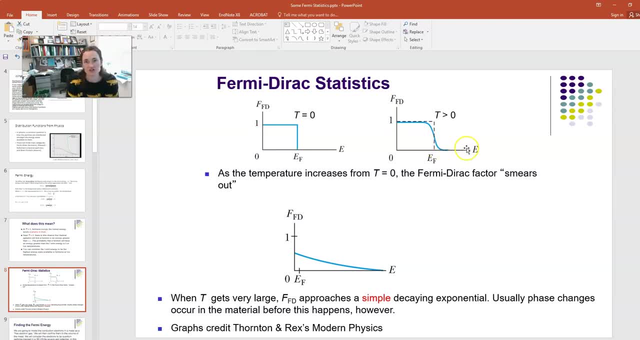 off, and what that means is that if you're above the Fermi energy right for t, greater than zero, there's a chance that you'll have higher energy states occupied right. So as it heats up, you can have energies greater than the Fermi energy, and as it heats up more, you'll get more there. all right, 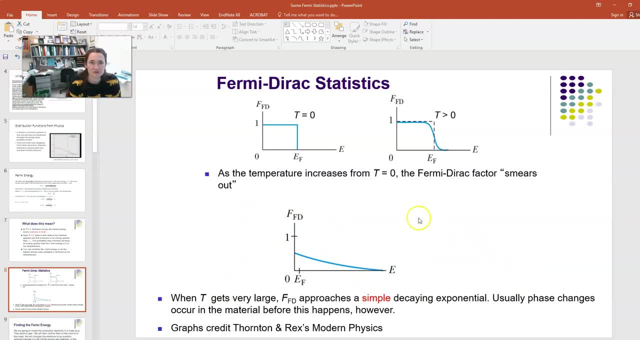 If it gets really large, then it's going to look like a simple decaying exponential. but I've got to tell you that this happens at really really high temperatures and you're probably going to have phase transitions of your material before your distribution function looks like that. So at reasonable temperatures. this will happen at really really high temperatures and you're going to have phase transitions of your material before your distribution function looks like that. So at reasonable temperatures. this will happen at really really high temperatures and you're probably going to. 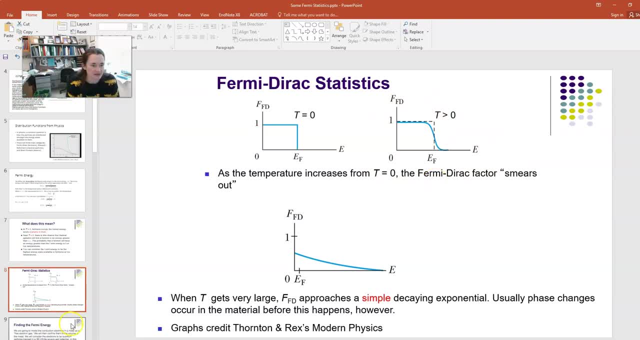 have phase transitions of your material before your distribution function looks like that. So, at rounded-off, distribution function is more along the lines of what we're thinking. Okay. so how do we find an expression for the Fermi energy? Well, we're going to model the 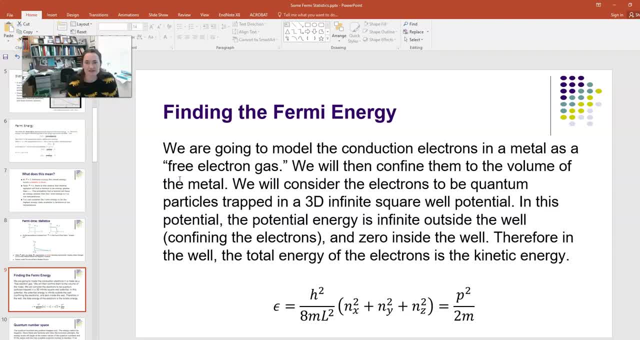 conduction electrons in a metal as a free electron gas. So what we're going to do is we're going to confine them to the volume of the metal. So you can think of them as being in a box, right, An infinite square, well, three dimensions, right, And it's trapped. They're trapped in that box, So in that. 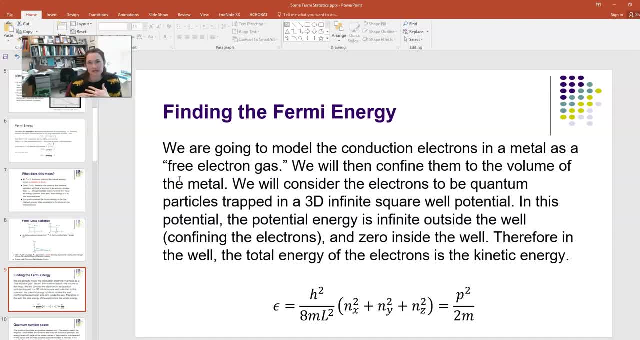 well, the total energy of the metal is going to be the volume of the metal- So you can think of them as electrons- is going to be the kinetic energy because, remember, for our infinite square well potential, we model the potential as infinite outside of the well, but inside the well we model. 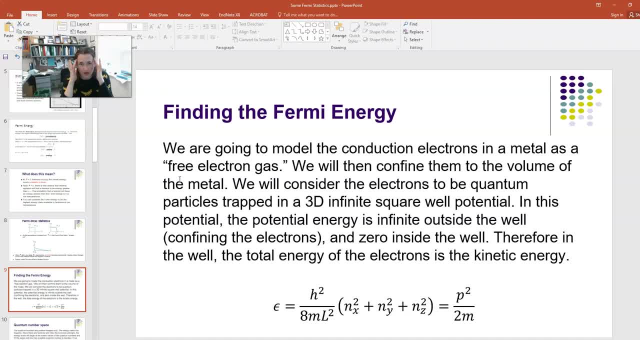 it as zero. So this is. you should think of your quantum square well, right here. So basically, remember, in a previous lecture we covered what the energy states were for a particle confined to an infinite square, well, in three dimensions, and that's described by this function here. 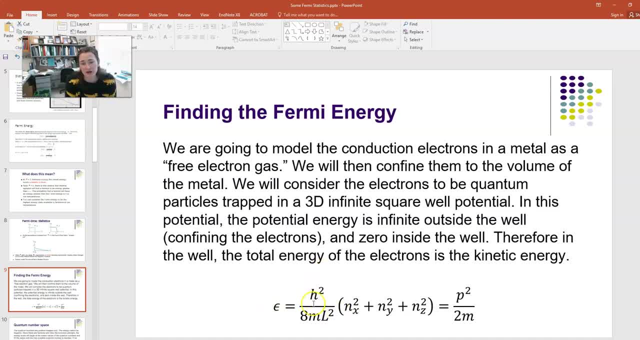 The energy is lost in the energy state of the energy state of the energy state. So this is: is equal to h squared over 8 times m times l squared times the sum of the squares of the quantum numbers in each dimension, which is nx squared plus ny squared plus nz squared Now here. 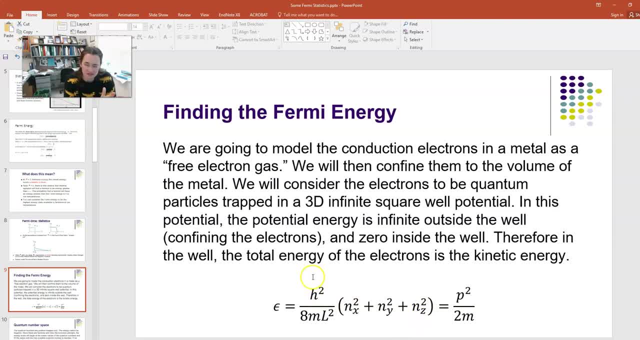 h is Planck's constant, which is 6.626 times 10 to the minus 34. in SI units, The m is the mass of the particle that's confined. so here that would be the mass of an electron, which is 9.11 times 10. 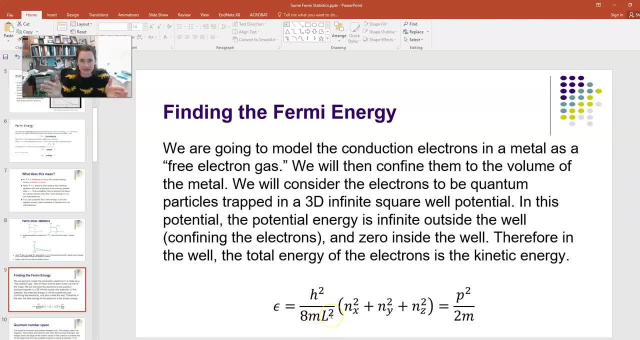 to the minus 31 kilograms. and then l is the length of the well, right, so it's how long the well is in that one direction. We're assuming here that it's a cube, basically. so it's confined and it's got l on all sides. Now this is the energy, and inside of the well it's going to be all equal to the. 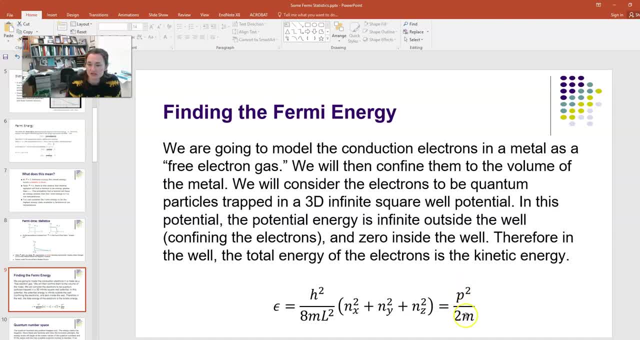 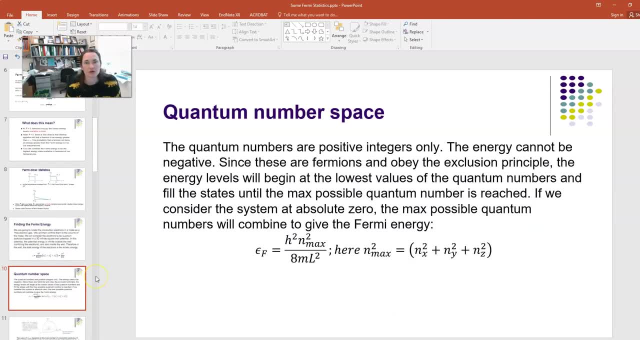 kinetic energy. Kinetic energy, remember, can be written as p squared over 2m, where p is the momentum of the particle. Okay, so three-dimensional, infinite energy. Now remember that these quantum numbers, for the 3d square well, are positive integers, only They. 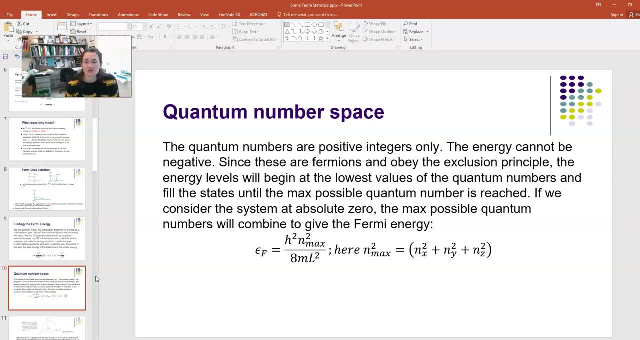 start at one and go up an integer steps from there, so the energy can't be negative. Now these are also fermions and they obey the exclusion principles. so what that means is that the energy levels are going to begin at the lowest values of the quantum numbers, and then they're 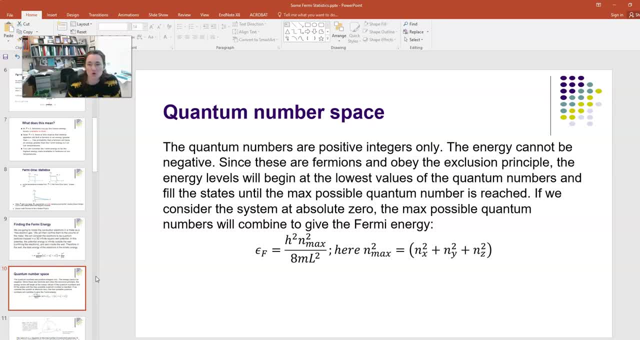 going to fill those states until the maximum possible quantum number is reached. So if we consider the system to be at absolute zero, we can draw that in this expression: it's going to be the maximum possible quantum numbers are going to combine to give that fermi energy right. So here we're, merging these two models. So 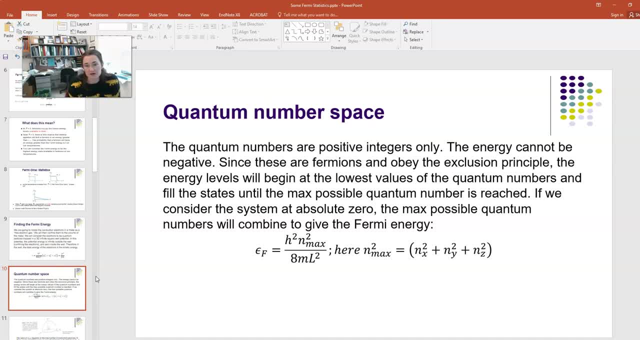 basically we can say that the fermi energy is going to equal to h squared times, what we are calling n max squared, divided by 8, n l squared. Now, here n max squared is going to be the squares, the sum of the squares of the quantum numbers for each direction. So n max squared is equal to nx squared, to total value of one nx squared. 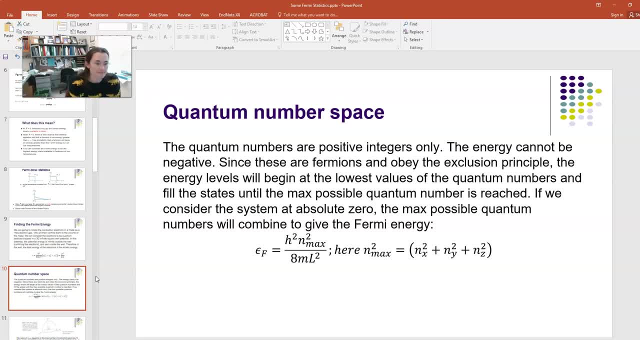 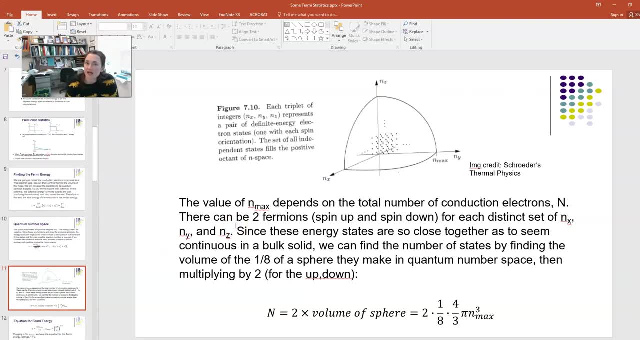 plus ny squared plus nz squared. okay, now, what would that look like? well, you've got only positive numbers. so if you wanted to plot this out- what it might look like in quantum number space- then you would have your x, y and z quantum numbers all plotted on each independent. 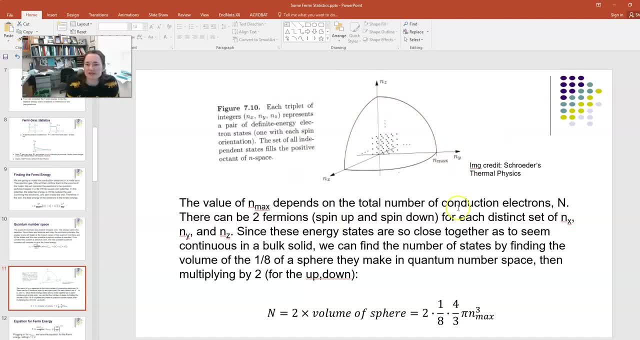 perpendicular axis. so this is quantum number space plot of it right here, with nx and y and nz. n max you could think of like the radius of this little section of the sphere, if you'd like. okay, now the value of n max is going to depend on the total number of conduction electrons that you have. 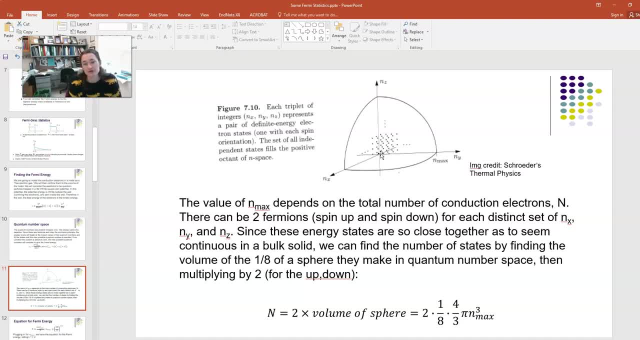 which i'll call big n. okay, remember that there can be two fermions, one spin up and one spin down, for each independent, distinct set of nx, ny and nz, and that's because of the, you know, poly exclusion principle. so you have these energy states. they're going to be really close together, right, Because you've got so many. 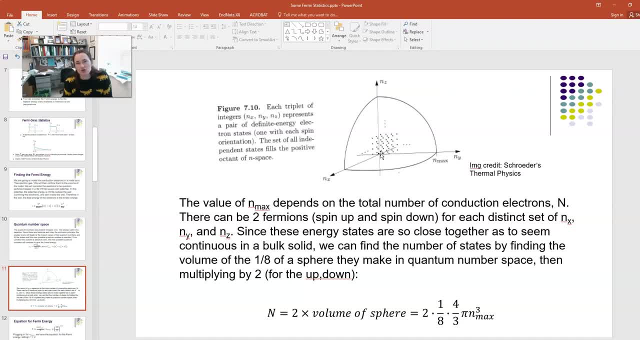 conduction electrons, that these energy states are going to look really close together, So we're going to assume that they start to look continuous. Now this model does break down, and I'm going to talk about that later, But for now let's go with it, okay? So they're going to seem continuous in. 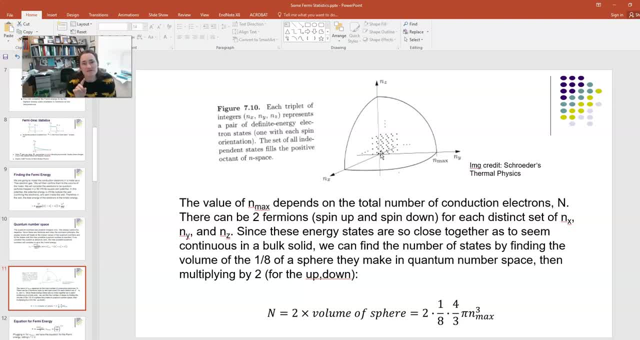 a bulk solid. So we can find the number of states by finding the volume of that one-eighth of a sphere that we've got here in our plot as they make up in quantum number space. And then we're going to multiply that volume of that sphere in quantum number space by two to account for the 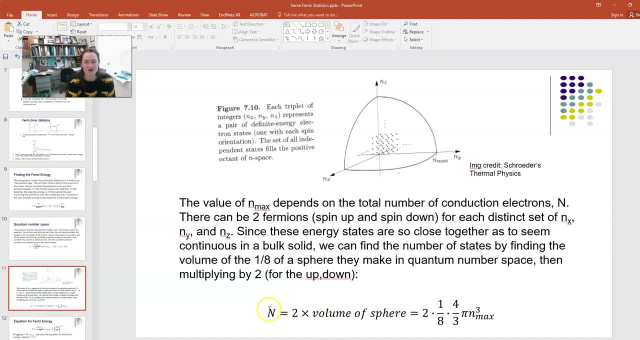 spin up and the spin down particles. okay, So here big N is two times the volume of my little one-eighth sphere here. So you've got one-eighth of a sphere. So the volume of a sphere of course is four-thirds pi r cubed right. So we have one-eighth times, four-thirds times pi, times n. 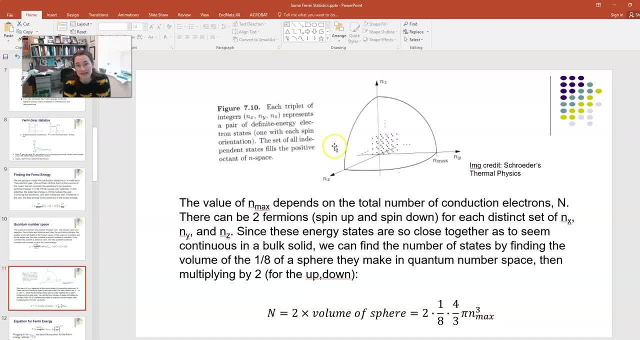 max, max cubed, Remember, we think of n max like we think of the radius of our little 1-8th sphere, And then we multiply that by 2 because we've got a spin up and a spin down for each quantum state. 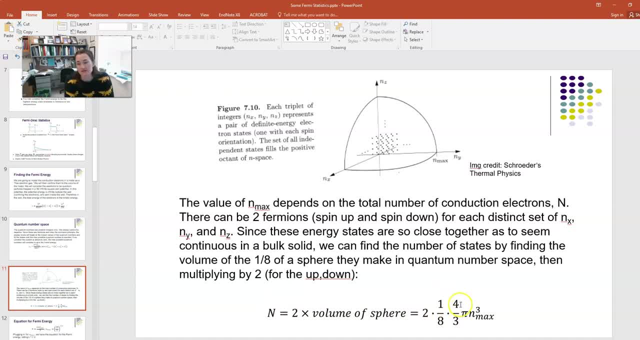 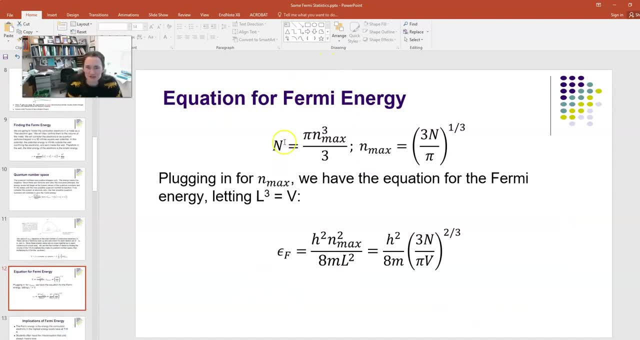 So that gives us big N is equal to 2 times 1-8th times, 4-thirds times pi n, max cubed. Okay. so how am I going to get a Fermi energy out of this Right? all right, here we go The number. 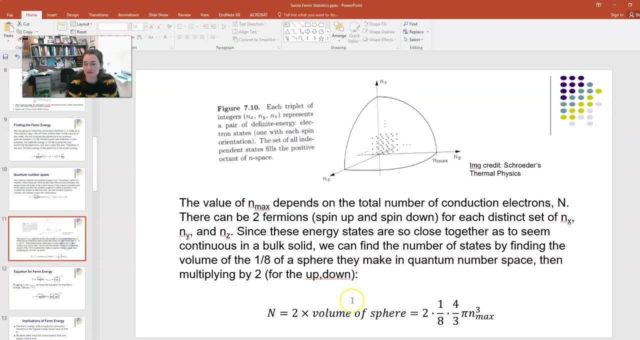 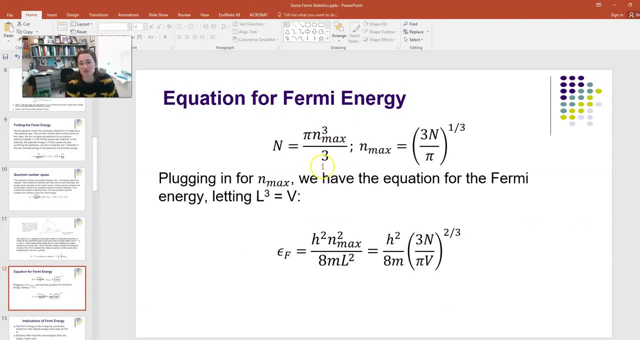 of conduction electrons. if I simplify this previous expression, here I have n times 2 times 1-8th times 4-thirds times pi n max cubed. right, We get some cancellation there. So the 8 cancels out with the 2 and the 4 on top and I end up with big. N is equal to pi n max cubed over 3.. 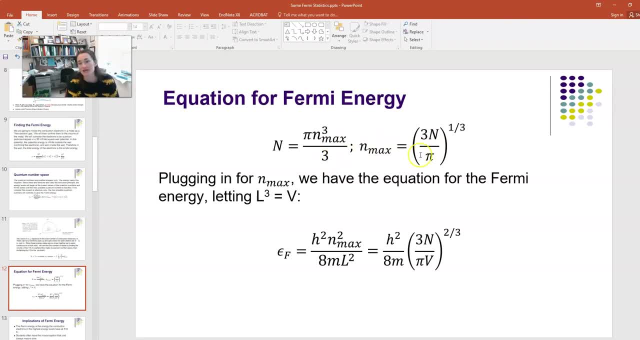 Now I can solve for n max right using this equation. n max would be 3 times big N over pi to the 1-third power right taking the cube root there. Now I'm going to plug that equation in right, plugging in for n max, into our equation for the Fermi energy. We said that the Fermi energy 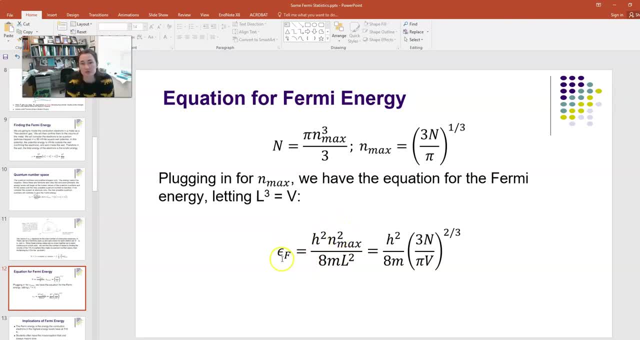 should be proportional to this infinite square. well, energy, which we said was h squared times n max squared over 8n, l squared right. So if I plug in for n max, I've got the n max is equal to 3 over pi, to the 1-third power right. And then I have this l squared on the bottom here. 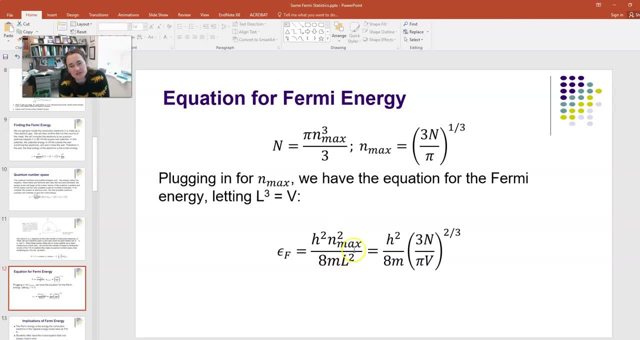 So I have an n max squared over l squared. So if I pull both of those inside, this 1-third root bit here, then what I end up with after a little bit of algebra. you can pause it here if you need to think about the algebra, that's h squared over 8n times 3n over pi v to the 2-thirds power. 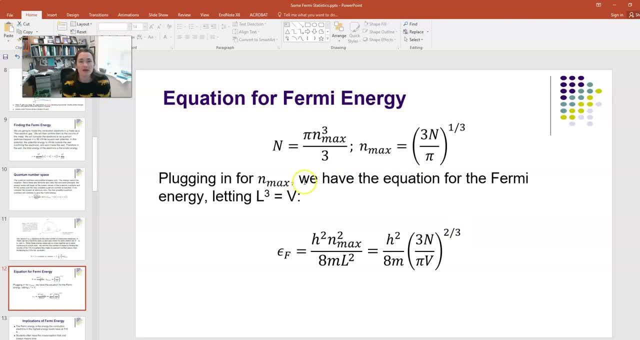 Now remember what's the v? V is volume and the volume of our 3d box. since it's a cube with sides, l would be l cubed. And see here: if I take 1 over l cubed to the 2-thirds power, I get l squared. 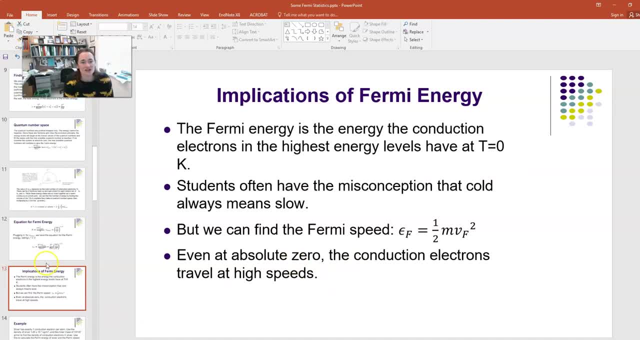 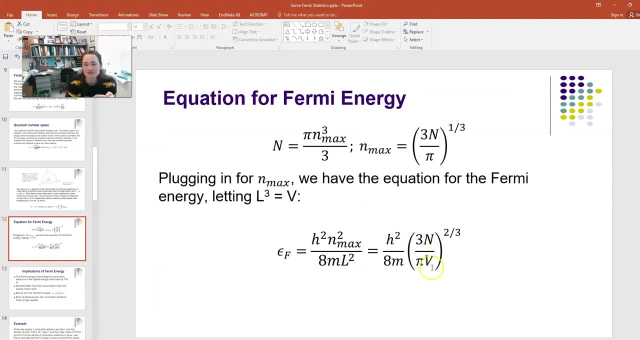 okay, All right. so that was our equation for the Fermi energy, all right. The Fermi energy was h squared over 8n times 3n over pi v to the 2-thirds power. okay, You can see there that it's mostly dependent. 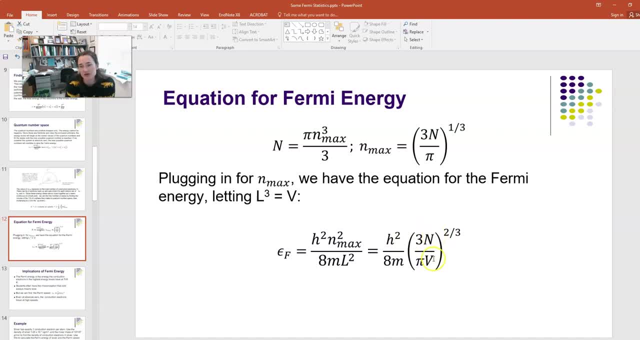 upon n over v, which is the number of conduction electrons per unit volume, and that's going to vary from material to material. So this is a material property, okay. So what is this? Fermi energy? It's the energy that conduction. 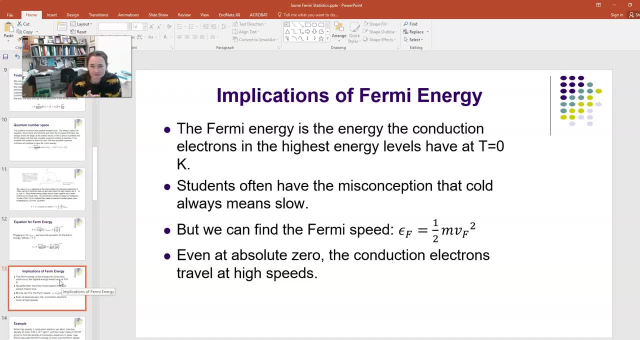 electrons in the highest energy levels have at zero Kelvin. Now here's another fun thing. Students often have the misconception that cold means slow and this comes from the ideal gas model. right, We say that in the ideal gas you have these atoms that are zipping around right at high speeds. 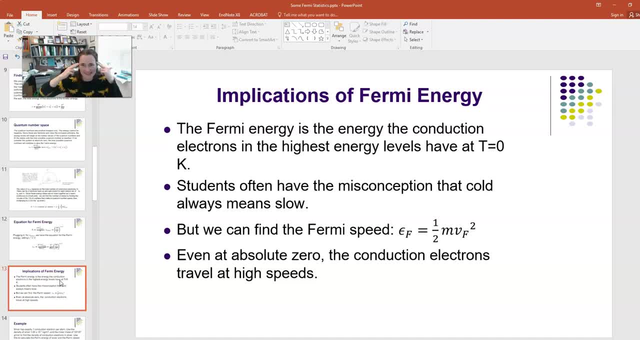 and then, as you chill it down, they get slower and slower. So that's the conception there. But not all particles are classical particles, are they? So these fermions aren't. They're not classical particles, They follow a difference. They're just a set of statistics So we can find how fast they're going, or at least a ballpark estimate of how fast. 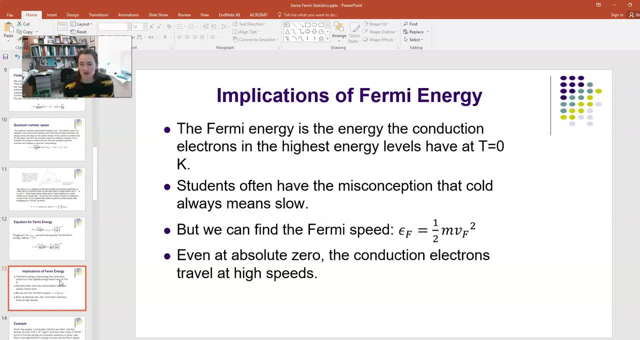 they're going by finding what's called the Fermi speed, So we can set the Fermi energy, which we have an equation for, equal to a kinetic energy. Say that that's one-half m v Fermi squared right, And then we can solve for v. 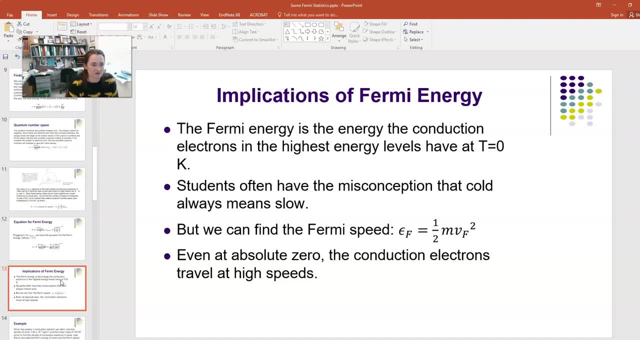 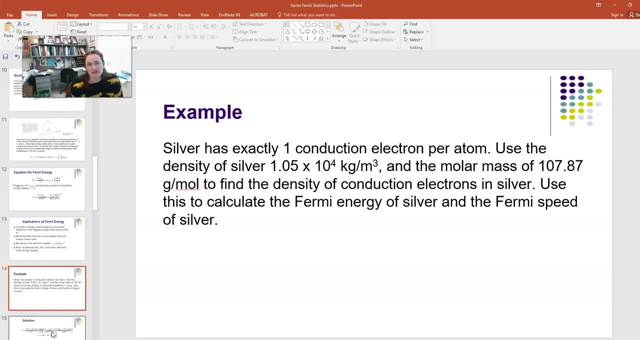 Fermi and find out a ballpark estimate about how fast they're going. So let's do an example problem of all this kind of cemented in our head. Silver donates one conduction electron per atom. So we're going to use the density of silver which is given as 1.05 times 10 to the 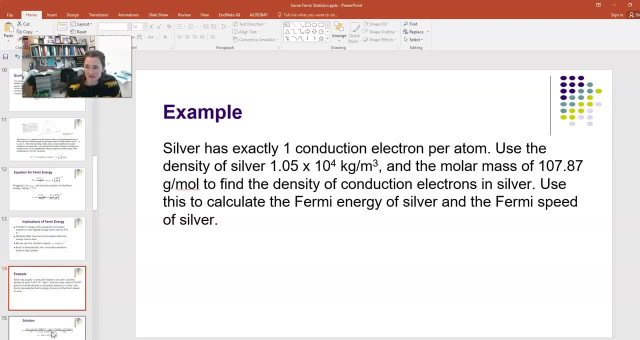 fourth kilograms per cubic meter, and the molar mass of silver, which is 107.87 grams per mole, to find the density of conduction electrons in silver, And then we're going to use that to calculate the Fermi energy of silver and the Fermi speed of. 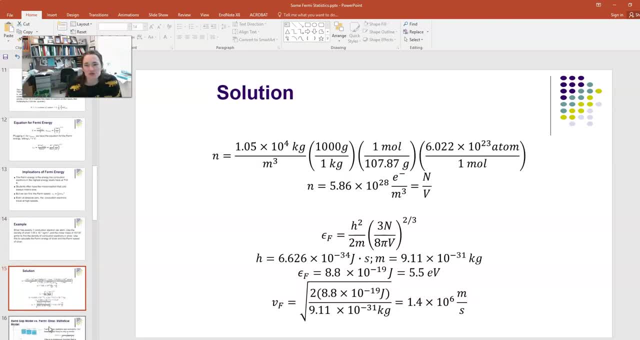 silver. So how do we do that? Well, you start off at a density and you basically just do a unit conversion. So silver has a density of 1.05 times 10 to the fourth kilograms per cubic meter. all right, 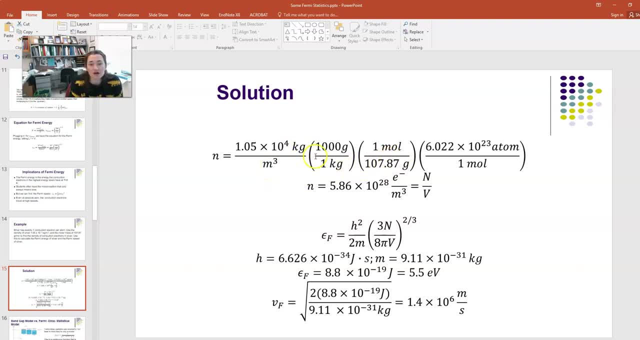 Now I'm going to go ahead and use that molar mass. So I'm going to convert from kilograms to grams- One kilogram has 1000 grams, right? And then I'm going to use the molar mass of silver. So one mole is 107.87 grams. So I multiply by 1000, I divide by 107.87,. 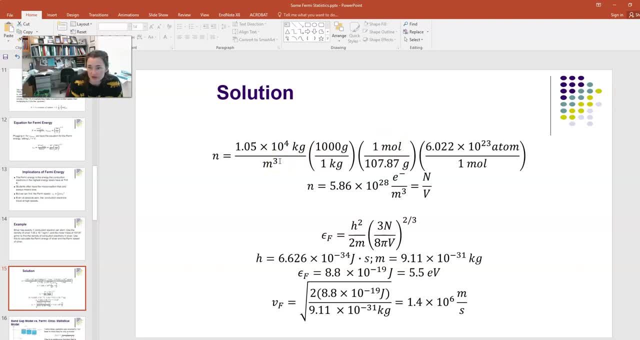 then I have the number of moles of silver per cubic meter. But I don't want moles of silver, I want number of conduction electrons. So first I'm going to convert to the number of atoms per cubic meter, right 6.022 times 10 to the 23rd atoms per mole, And when I do that I end up with a density of 5.86 times 10 to the 28 silver atoms per cubic. 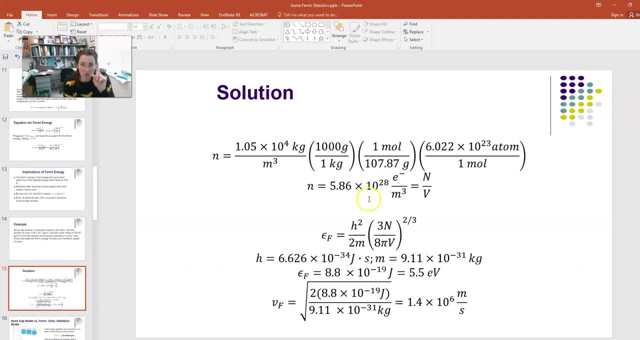 meter. Well, each silver atom contributes one conduction electron. So that means that the density of conduction electrons is actually 5.86 times 10 to the 28 conduction electrons per cubic meter. Now that is going to be n over v big, N over v right, And that goes into our 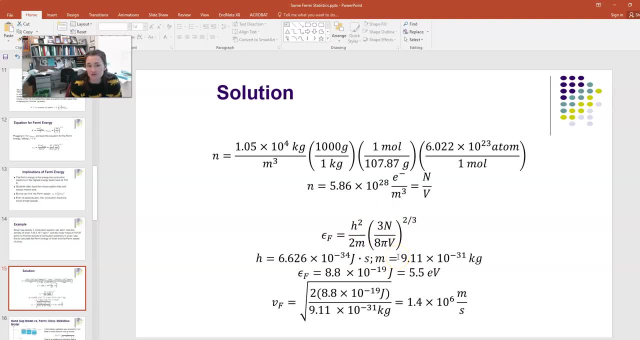 formula for our Fermi energy. The rest of our Fermi energy formula is just fundamental constant. We've got H, which is Planck's constant, and we've got the mass of the conduction electron, which is 9.11 times 10 to the minus 31 kilograms. So plugging all that into our calculators, 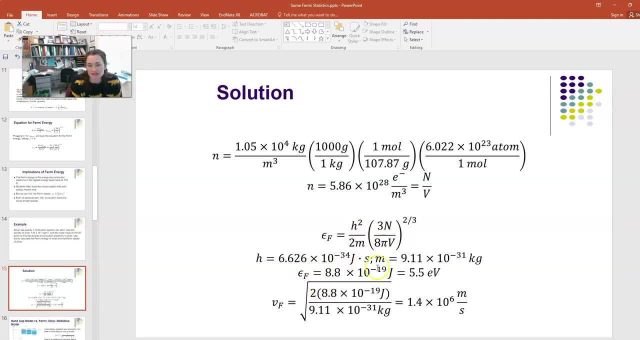 right, we end up with a Fermi energy of 8.8 times 10 to the minus 19 joules, Doing a conversion from joules to electron volts, which is a more convenient unit, quite frankly, for a Fermi energy. 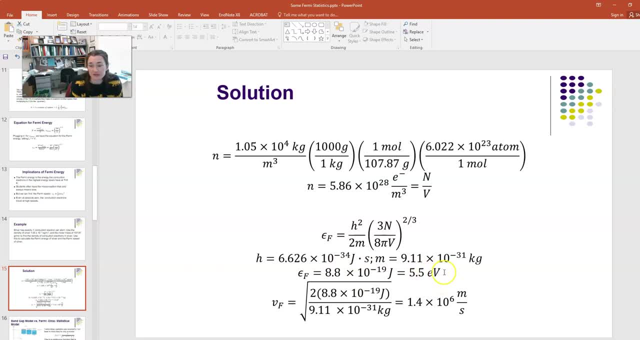 we end up with 5.5 electron volts for the Fermi energy of silver. Now that we have the Fermi energy right, we can use that to find the Fermi speed. You said the Fermi energy equal to 1 half. 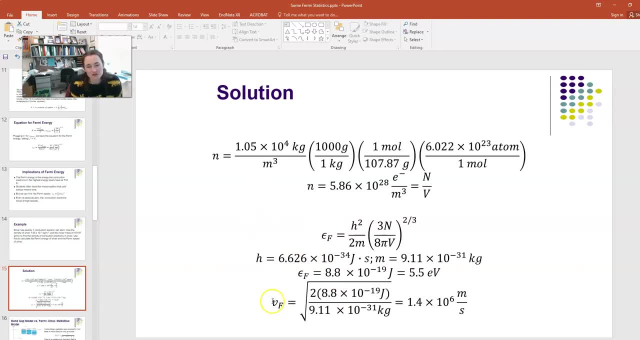 m v Fermi squared right. So you can find the Fermi speed by taking the square root of 2 times the Fermi energy divided by the mass. Doing that here, I see that the Fermi speed of silver is 1.4. 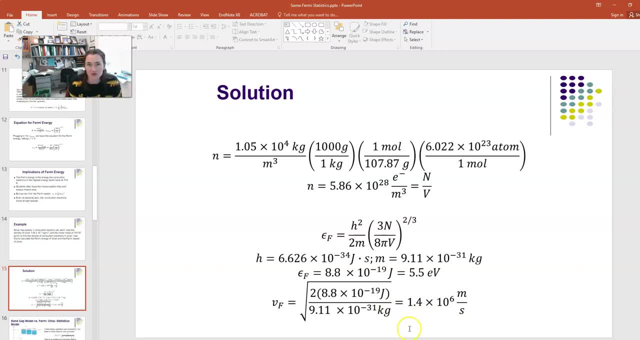 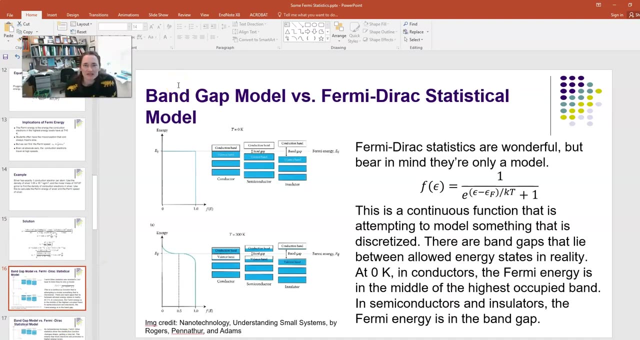 times 10 to the 6 meters per second. So that's not slow right? That's like 0.3 percent of the speed of light, So it's going pretty fast, Even at very low temperatures. Now, what does this all mean in terms of what we learned before? 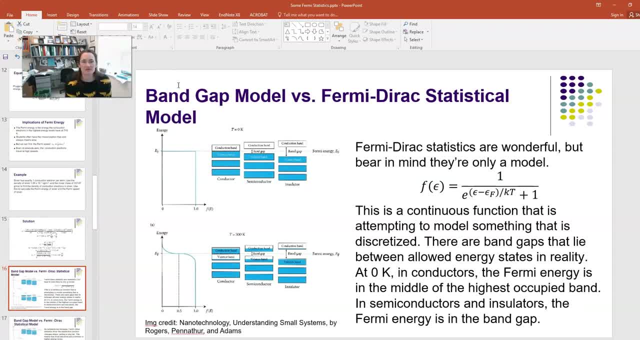 about band gaps, okay. So let's think about the band gap model and contrast that to this Fermi-Dirac statistical model for just a second. So here I want to tell you this: Fermi-Dirac statistics are wonderful, but you have to bear in mind it's only a model. and what are the 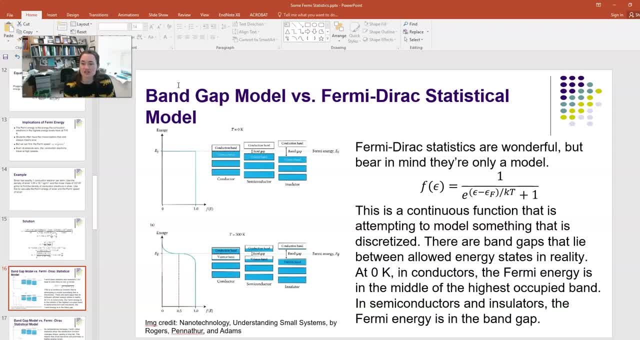 limitations of that model. So the Fermi-Dirac function is only a model, and what are the limitations of that model? It's a continuous function. Now it's attempting to model something that's discretized, but it makes a big assumption there and it says that we're going to assume that. 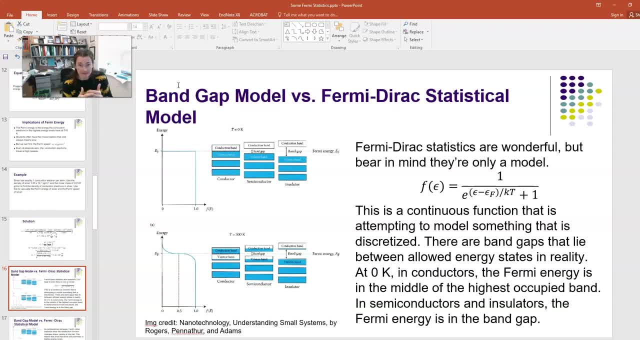 the energy states are close enough together that they look continuous, and that was an assumption that we made way back at the beginning and that's not actually true. okay, We know from our band gap model that we discussed in a previous lecture that there's actually allowed bands of energy. 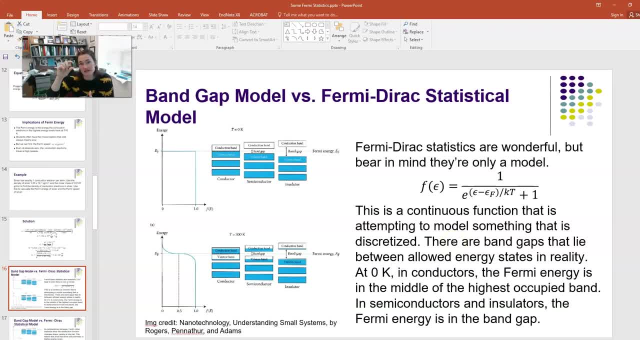 states and that in between those allowed bands of energy states there's gaps, band gaps, right? So if you were to take the Fermi energy kind of model and map it over onto the band gap model, this is more like what you would see up here in the top portion of this figure as the temperature. 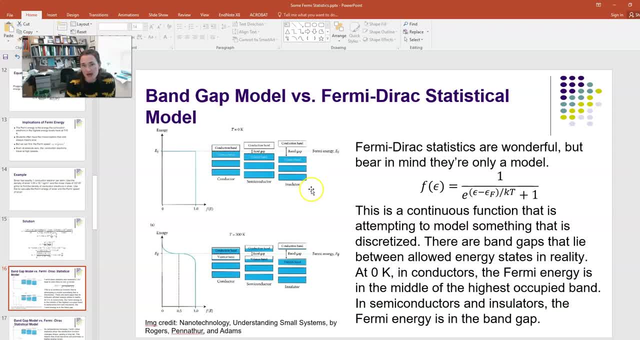 approaches zero Kelvin. Remember that what we said was that zero Kelvin is the maximum possible allowed energy state. right, That's max possible. What would that mean to take it over into our band gap model? Well, what it would mean is that for conductors it would lie kind of in the 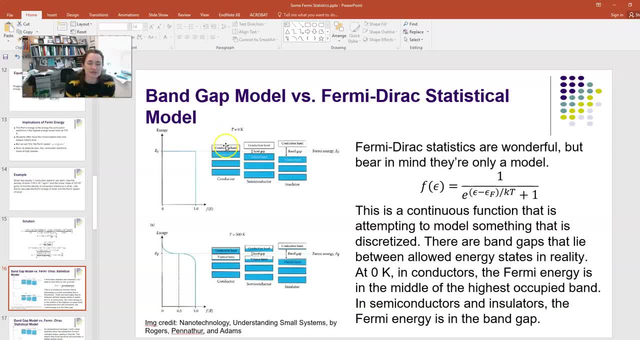 middle here of this valence band in the conduction band and you can see that at zero kelvin there's not a lot of electrons in the conduction band but there are still some. and as you promote more and more, as it gets hotter and hotter, you're going to fill that conduction band more and more. but 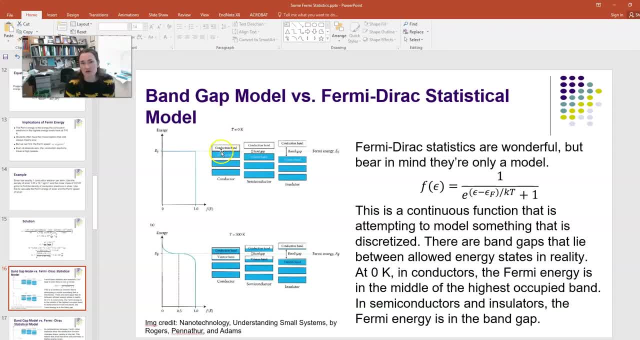 for a metal, even at zero kelvin. you've got some uh electrons that are uh in that conduction band and so you can see here this dashed line right here represents the fermi energy, and you can see that you've got this kind of purple region here where you've got some electrons that are in that. 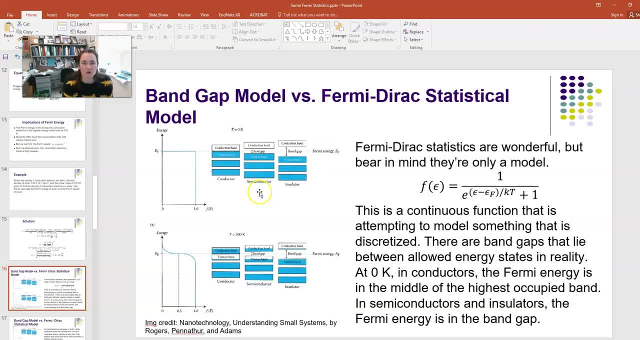 conduction band. now for semiconductors. what happens is that, uh, there's a band gap in between the valence band and the conduction band, and for semiconductors, the fermi energy lies in the gap in between the valence band and the conduction band. so that means that semiconductors really 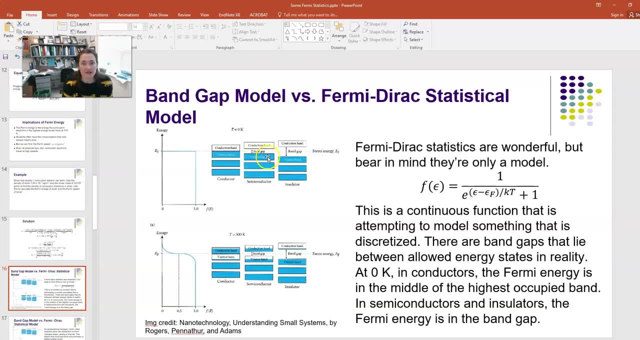 don't have anything as zero kelvin. that is above the fermi energy and there really is that gap there. okay, and so when we go up to the valence band that's going to show up and we're going to, and all the ones underneath are occupied states.